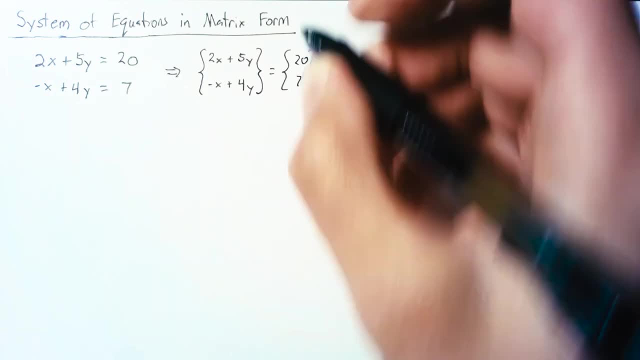 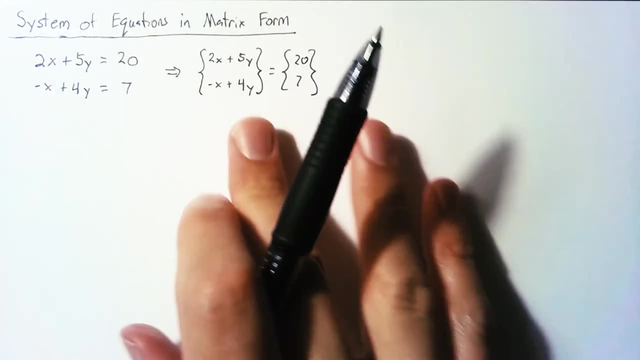 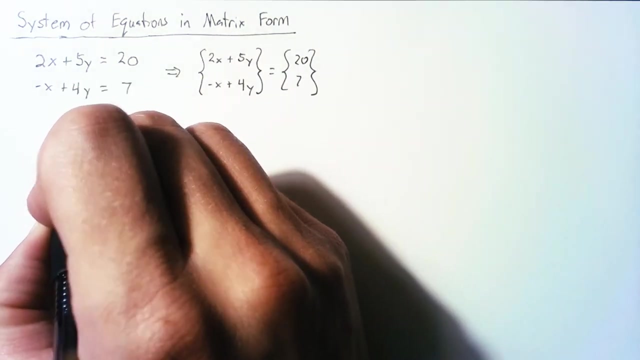 So each of their elements needs to be equal, which means that this equation is the exact same thing as this system of equations. Now, to move on from this, we need to remember some of the rules of matrix multiplication, because what we want is a matrix that is going to be multiplied by 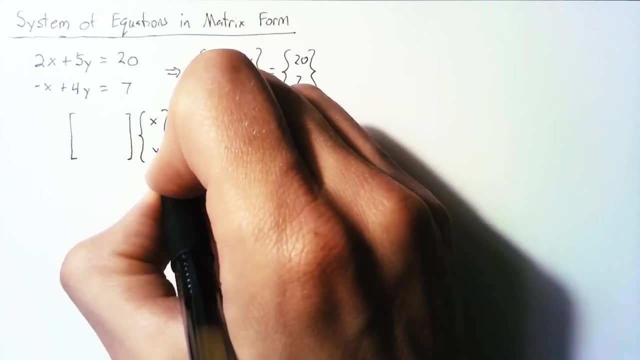 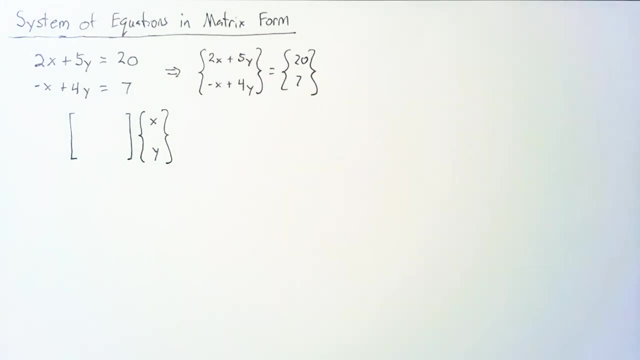 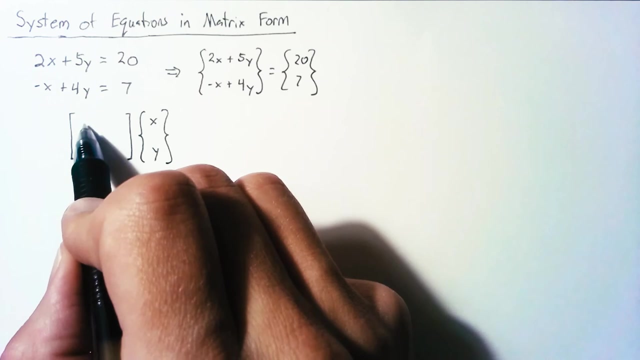 our unknowns. So our unknowns are x and y, and we want a matrix that we can multiply this by. We want a matrix that is going to be equal to this element multiplied by x, plus this element multiplied by y. Really, all we need to do is put the x value here and the y value. 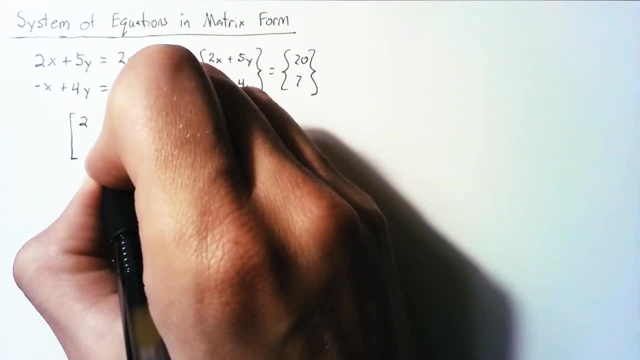 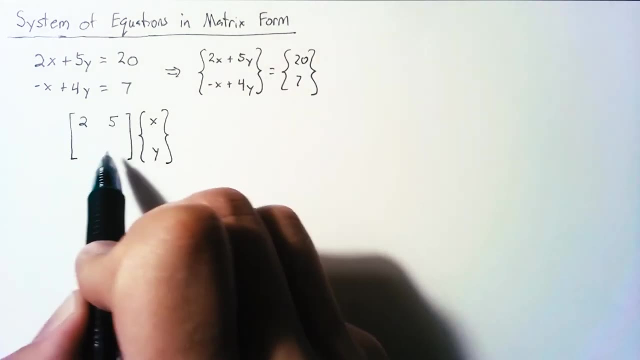 here, And it helps to think of the first column as the x column and the second column as the y column, And each row will be its own separate equation. So what we're going to do is we're going to put this x column as the x column and then we're going to put this y column as the y column. 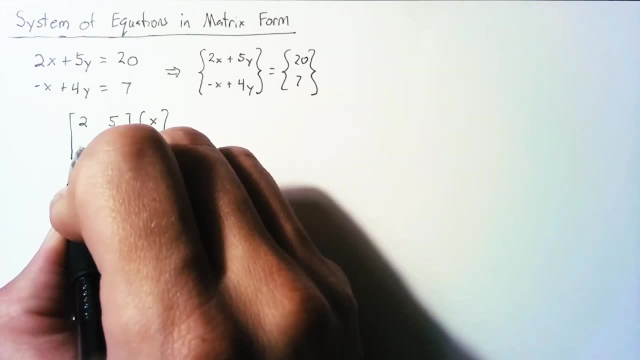 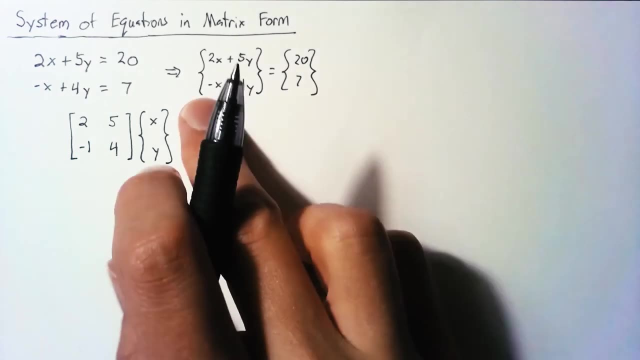 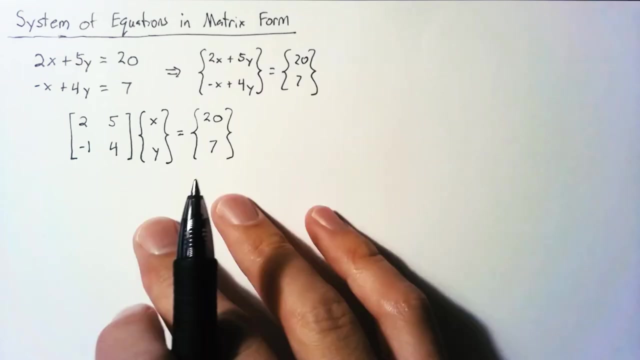 So our second row: here we take the negative 1 in the x column and the 4 in the y column and we can write those two in, and we'll end up with the second element of our vector, And so we're just going to leave that as 20 times 7.. So this is the matrix form. 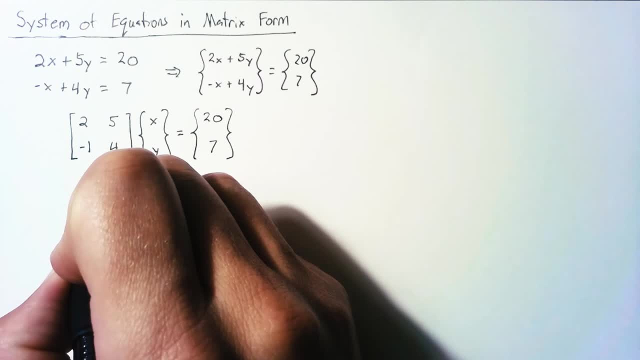 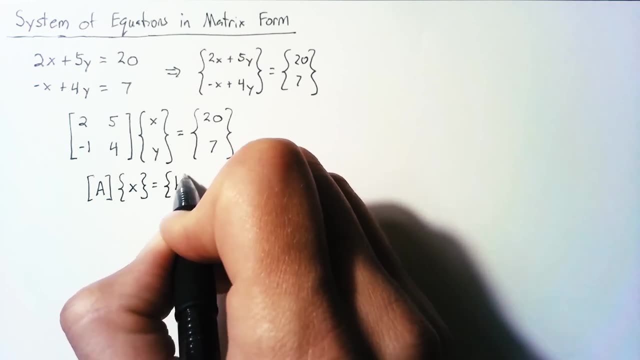 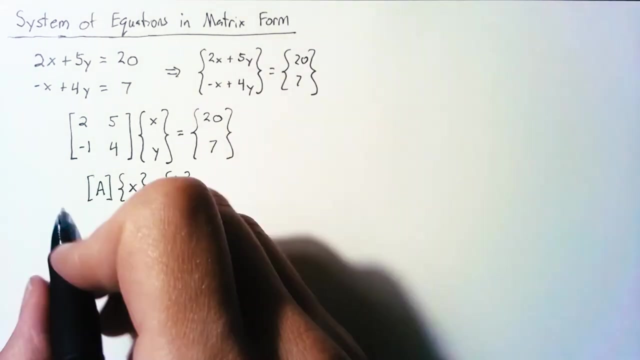 of our system of equations And a lot of the time. we're going to write this as some matrix A multiplied by some vector x, which is going to be equal to some vector b. ax equals b is our standard form. Now how do we actually solve this? 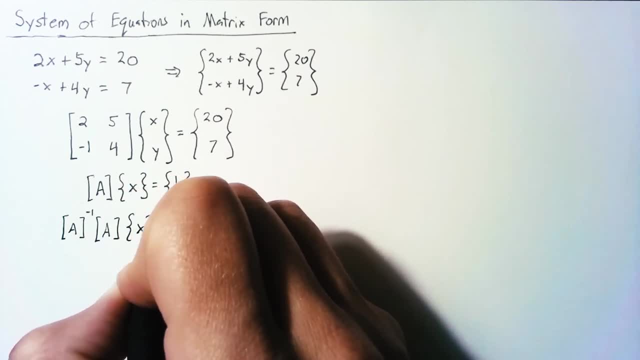 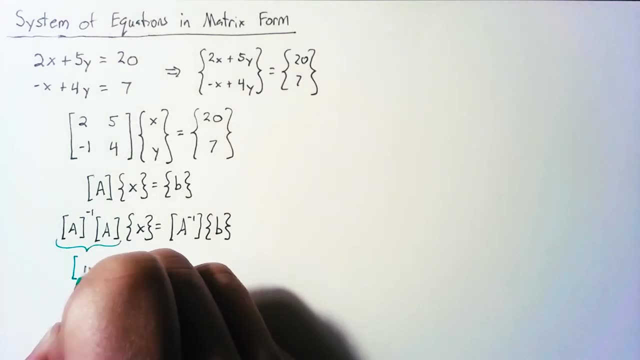 We pre-multiply both the left and the right-hand side by the inverse of A. So what happens here? our A inverse and A together become an identity matrix. The identity matrix multiplied by x just becomes x. So i multiplied by x is simply equal. 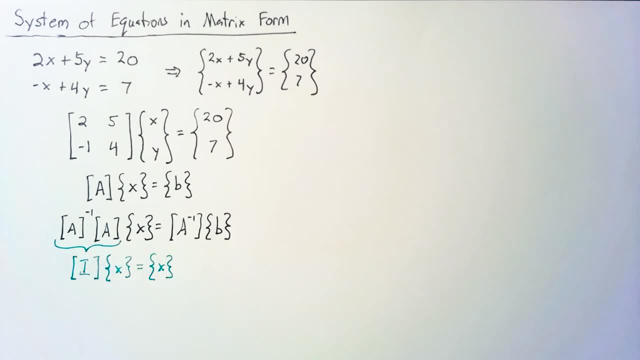 to x. So the effect of pre-multiplying by the inverse of A removes that A matrix. So the equation that we end up with is our vector of unknowns: x is going to be equal to the inverse of A multiplied by b. So how does that relate to our system of equations up above? 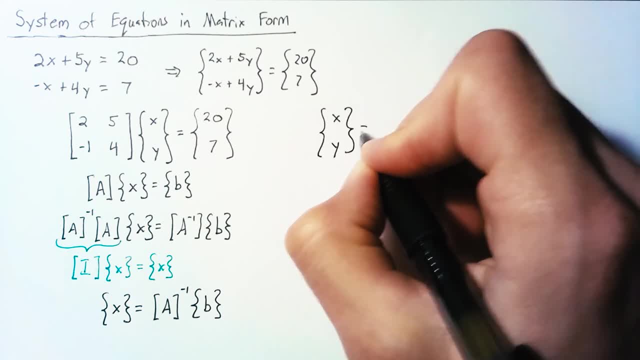 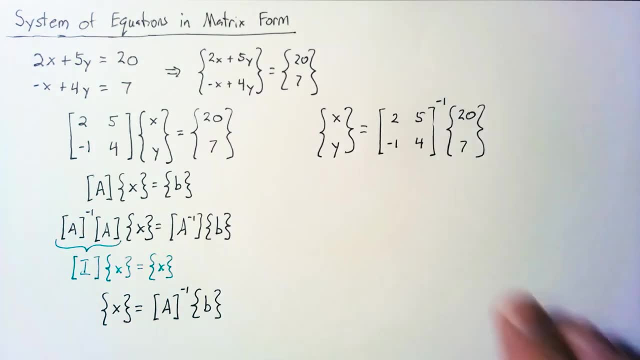 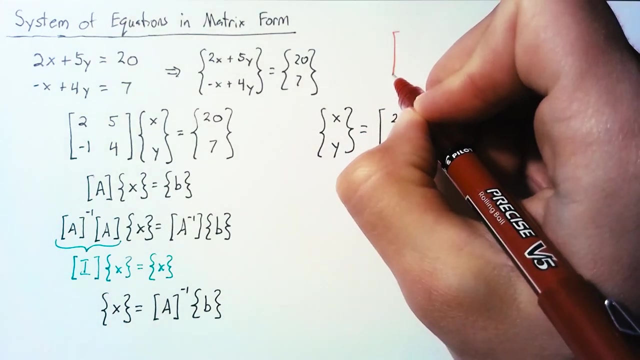 Well, it says that x and y are going to be equal to the inverse of our A matrix multiplied by our b matrix. So, as I said in the previous video, we have a way of calculating this directly by hand, And the formula that we get for that is: 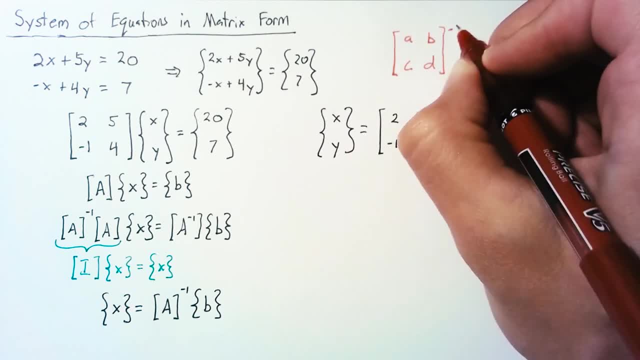 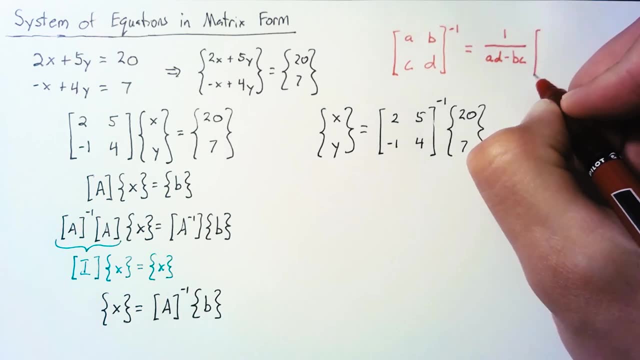 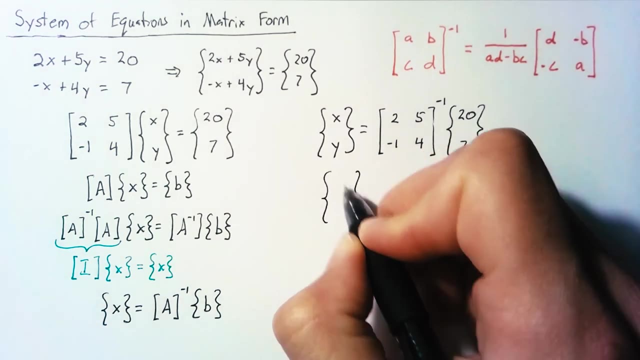 that the inverse of a matrix that has some coefficients is going to be equal to 1 over something called the determinant multiplied by d negative, b negative c and a. Applying that to our problem here we're going to end up with: 1 over ad is just 2 times 4,. 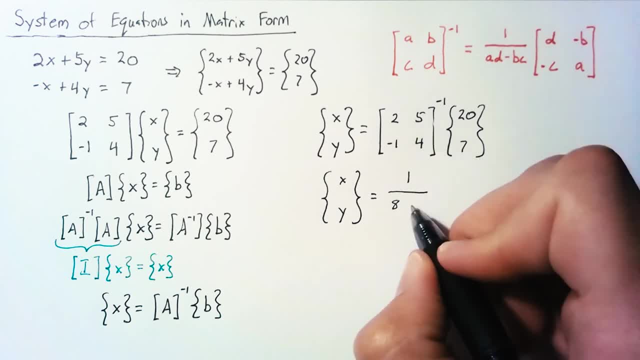 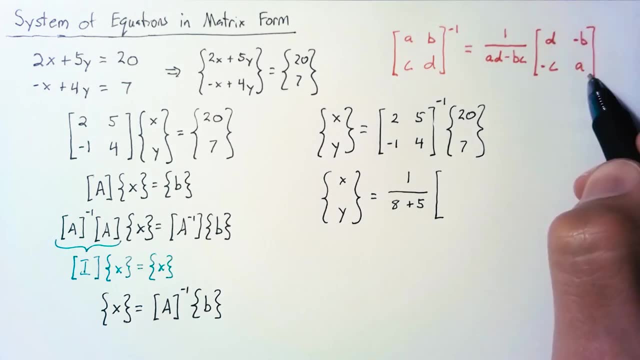 so that'll be 8, minus bc. that's a negative 1 times 5, so we'll have plus 5, multiplied by this new matrix. So we're swapping the position of a and d, so this will be 4 and 2 along the. 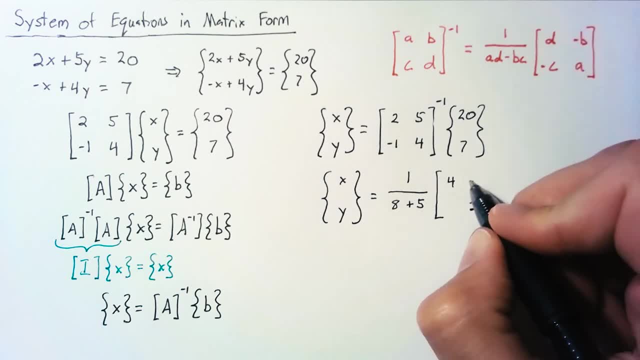 diagonal, And then we're just taking the negative of the b and c. so this will be negative 5 and positive 1. And that's going to be multiplied by this 20 and this 60. So we're going to have a. 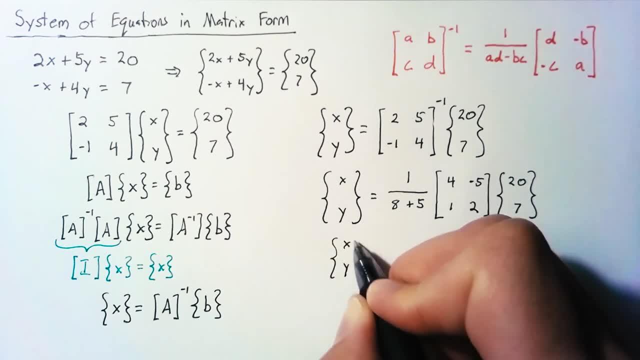 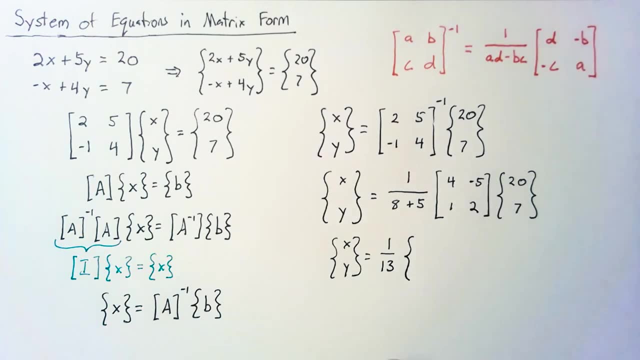 vector of this 20 and this 70.. So now what we can do is leave this 1 over 13 alone. but we're going to have a vector of two values which come from the first row multiplied by our column and our second row multiplied by our column. So our first row here says that we have 4 times 20, so this is: 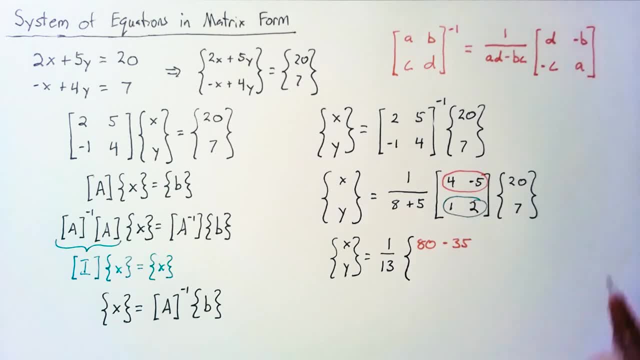 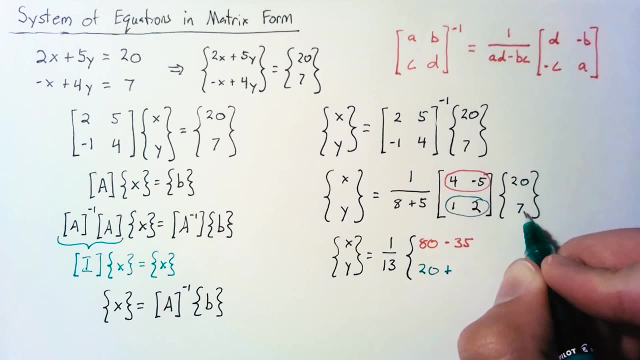 80,, plus negative 5 times 7,, which is going to be minus 35.. And then our second row. we have 1 times 20,, which is just 20,, plus 2 times 7,, which is 14.. 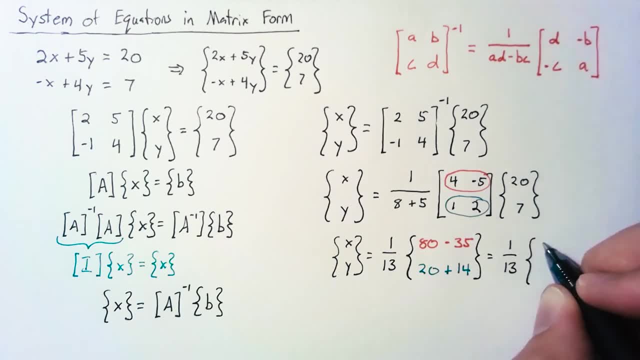 Putting that all together, we end up with 1 over 13, multiplied by 45 and 34.. And the way we interpret this is we say that x is equal to 113 times 45, and y is equal to 113 times 34.. 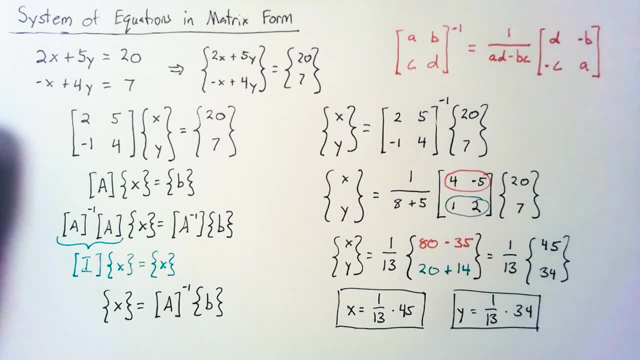 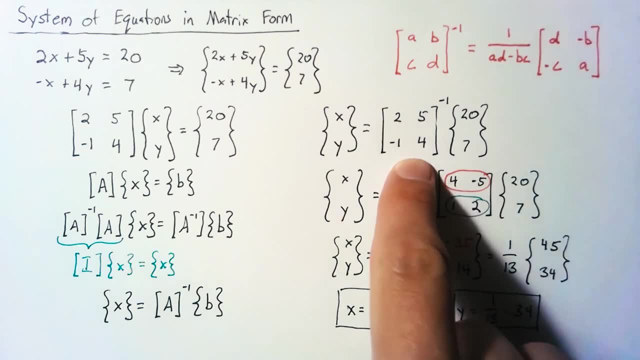 So this is how we write a system of equations in matrix form and go ahead and solve it. Now, the one thing that will change is we are rarely, if ever, going to be doing this by hand. This should almost always be done using a computational tool. 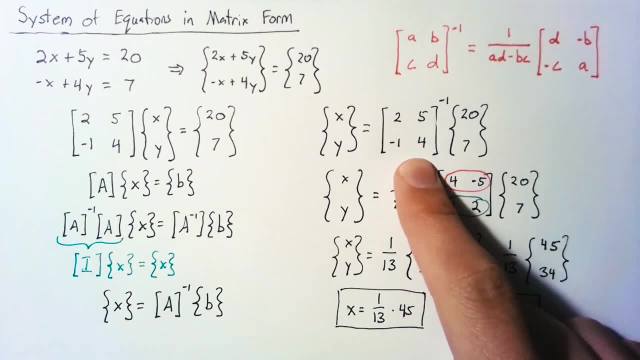 MATLAB and Python both have ways of doing this very easily, And if you don't have those available, then there are tools online that you can use regardless. So that is all we have for today. Thank you for watching. See you next time. 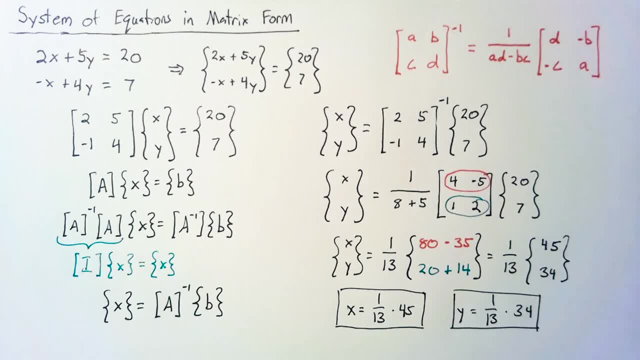 All for this lesson. I hope it was informative and I will catch you next time. 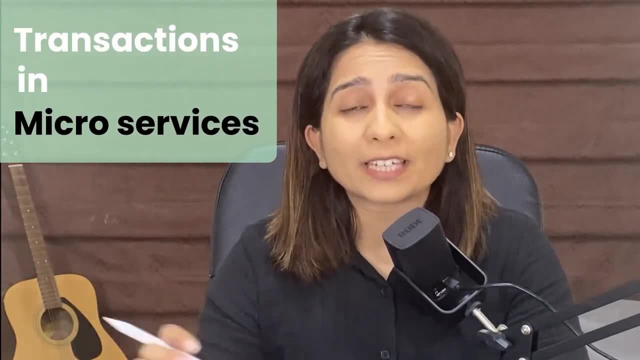 Transactions in microservices is another big problem and a complicated problem to solve. In today's video we will discuss the same and we'll also find out how it is solved in the context of microservices. When you have a monolith system, you just have one service- maybe your. 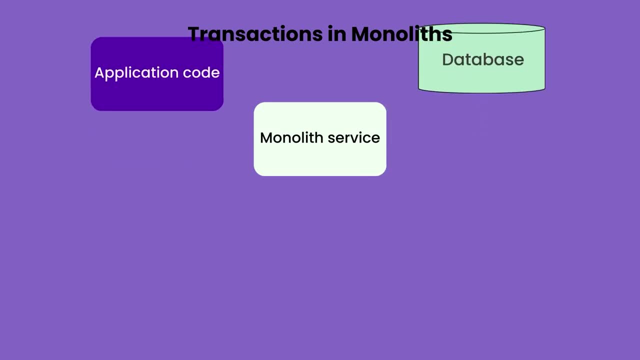 application code and your DB is deployed on the same instance. or you have one service and your DB is deployed on a separate instance. In any case, you have just one database. you have different tables Whenever there is a case when you have to make updates to two tables for one business flow. 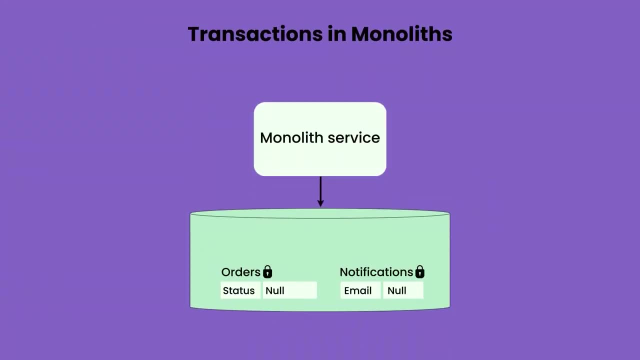 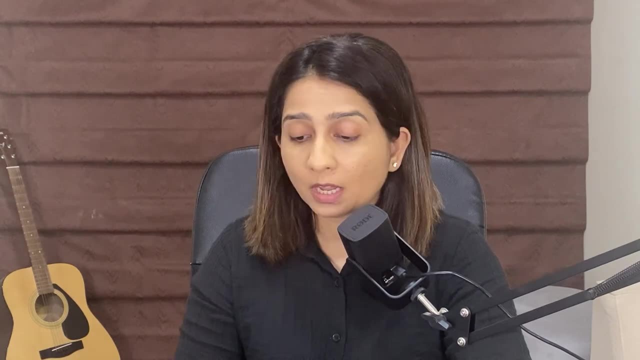 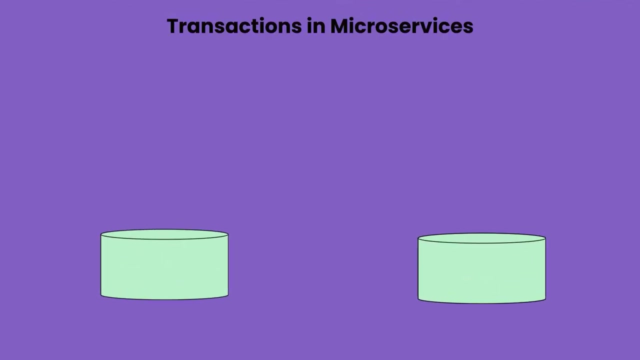 you just use a simple transaction: put a lock in both rows, update the rows and release the lock, and you are done. You commit the transaction. It is very easy. Now, what happens in the case of microservices? In the case of microservices, you have two different databases. you have two.